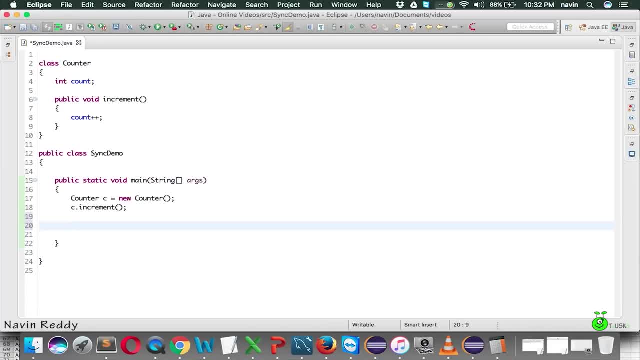 And later on let me create the object, I mean let me print the value of the count there. So we'll say systemoutprinter and we'll say count plus. we'll say this is c dot count, Is it? Yeah, So now, if I run, 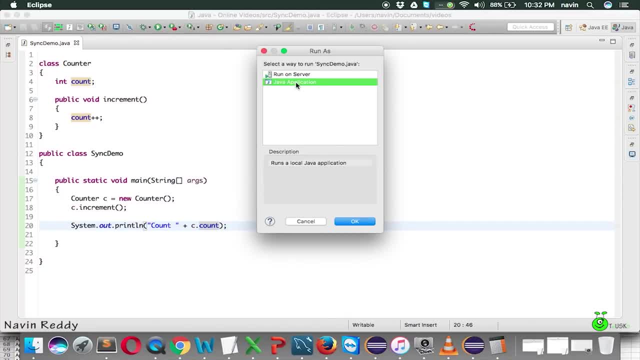 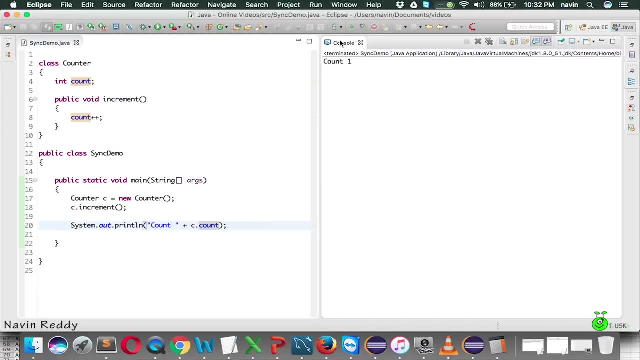 this code, you can see we'll be getting the output as. okay, so we got the output as 1.. So count is 1.. Let me take the output window here so that it will be very clear for us to see the output Now, since we are calling increment only once it is printing count 1.. What if I call increment? 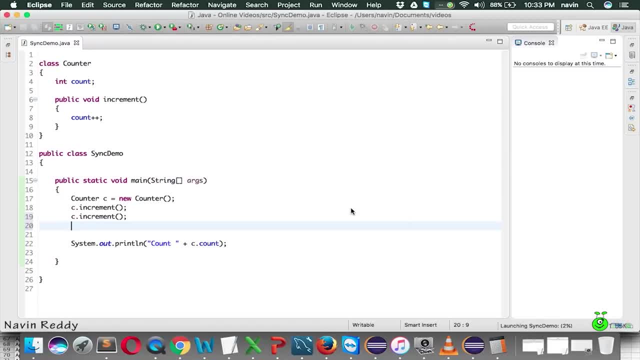 2 times. So it will run this and it will get. it will give the output which is 2.. Right, because we're calling increment 2 times. Now what I will do is I will call increment multiple times. So let me call increment, let's say, 10,000 times. Of course it's the count value. will be 10,000. Right, Okay, But instead of using count plus, I get 20 times. So I should have use count plusing change to a little less value And then call increment multiple times. So let me call increment, let's say, 10,000 times. Of course count value will be a much if at the comen 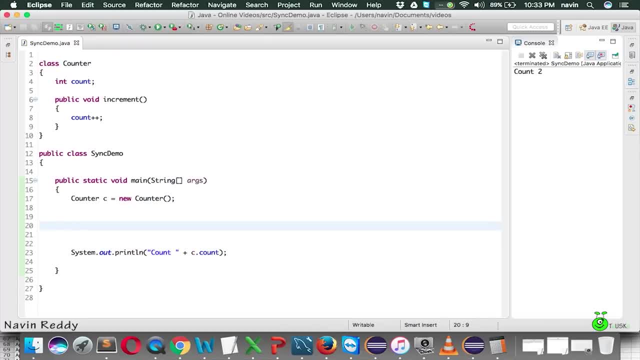 using main thread, I will count. I will count it for two, I mean it will. I will count using two different threads. so let's create a thread and each thread will call increment thousand times. let's do that so we'll say thread t1 equal to new thread. and now we know how to create the object. 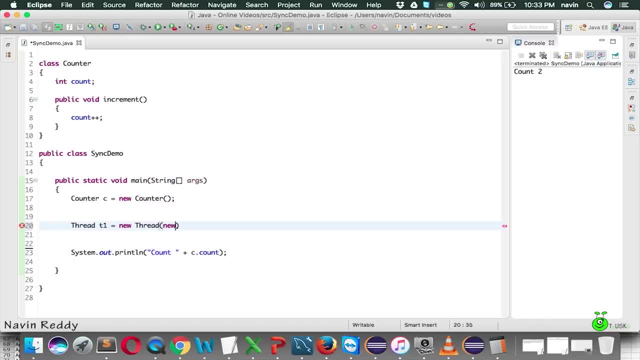 of thread, right, so we can use lambda expression here directly. but just to make it simple, I will be using runnable object. okay, I have, I want to create to, I want to. I wanted to create the object of runnable here and here I will create a method which is public, void run, which is compensative. 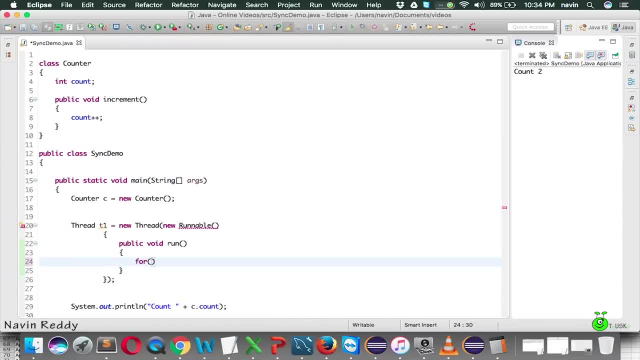 for us to do right. and then in here I will, I will run a loop which will start with one. it will go till one thousand, and then I will say plus, plus. so I got a for loop, so this for loop will run for 1,000 times, and every time it should call c dot increment. okay, so, 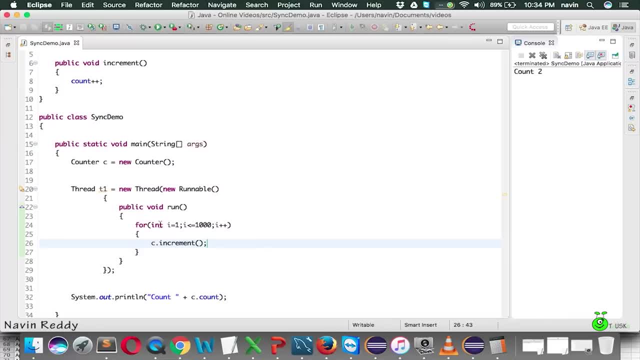 every time it should call c dot increment. Every time you call count, I mean every time you run this slope, it will call increment. So in total, the value of count will be 1000, right, Let's do that. Let me just say t1.start. 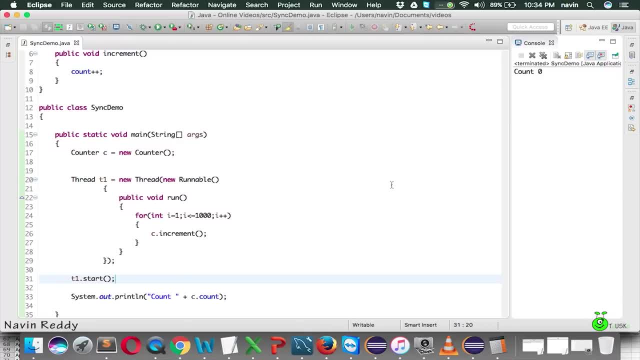 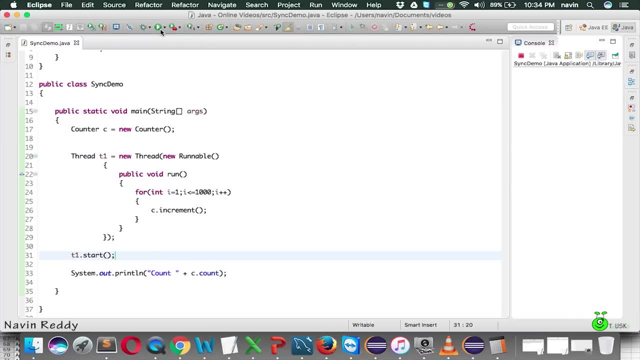 Will it work now? So I am using only one thread now And the count value is 0.. That's weird. Why it's not working? It's because it is working. If you can see, if you run this code, you are getting some value. You can see 0,, we got 219,, we got 205. 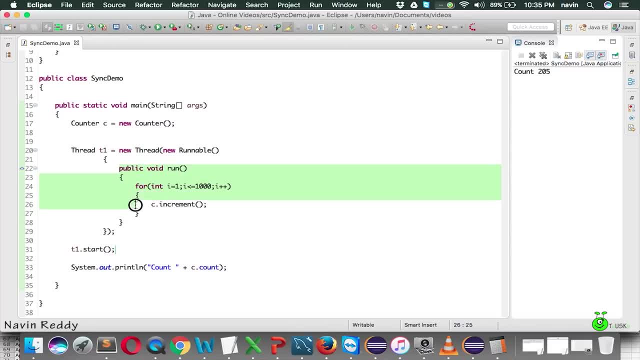 What is happening is, as soon as you say start, it is running this loop. It will take some time for running right. By the time, t1 is busy incrementing this. the main thread is doing nothing and it is printing the count here, right. 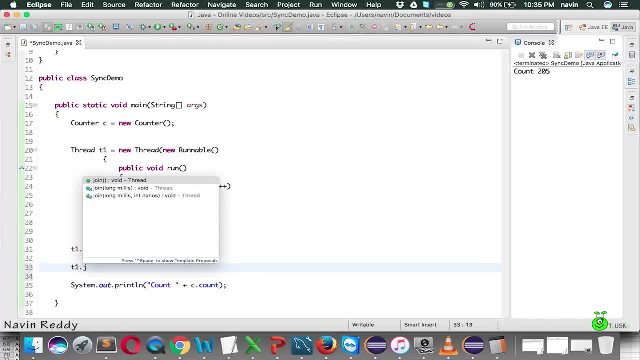 So what we will do is we have to ask our main just to wait for t1 to complete its job. So for that we have to say t1.join and it might throw an exception. It might throw an exception there. And now, if you run this, you can see: 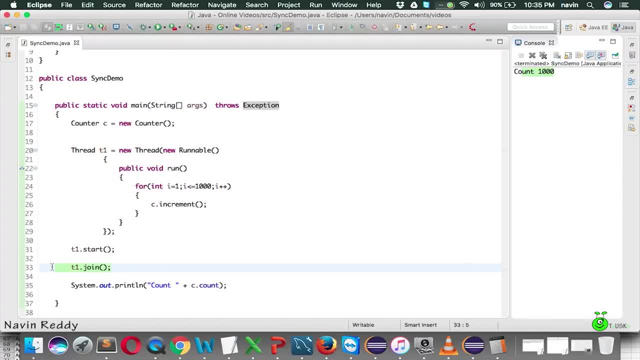 we got the count value as 100.. So what we are doing now with t1.join is we are asking our thread to wait. So we are asking our main thread to wait for t1 to complete its job. Okay, So that is only one thread, right. 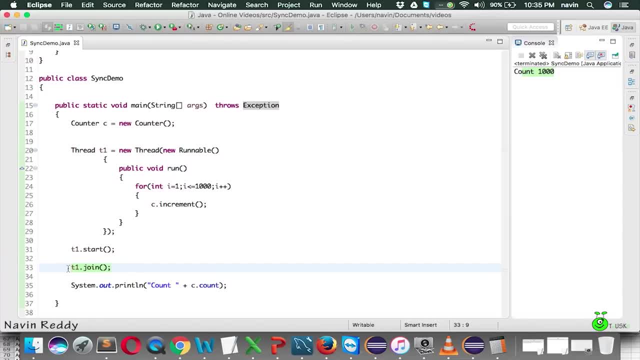 I want to use the second thread now. So how will you implement second thread? Let's see that. So let me just say so. let's say this is t1.done. Let me just copy this code and I will make one more thread here. 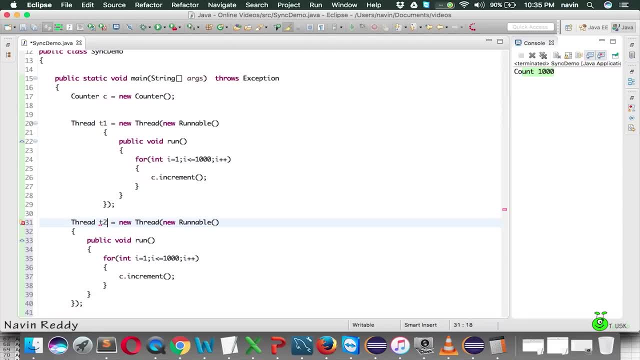 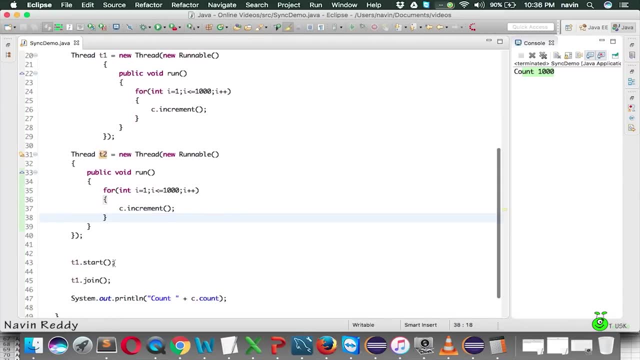 which is t2.. So we will make this as t2. And this will do the same thing. It will run this loop for 1000 times and it will call increment And we have to say t2.start, And then we have to also wait for t2 to complete its job, right? 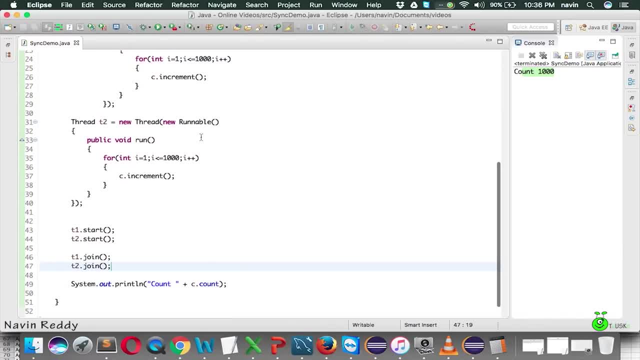 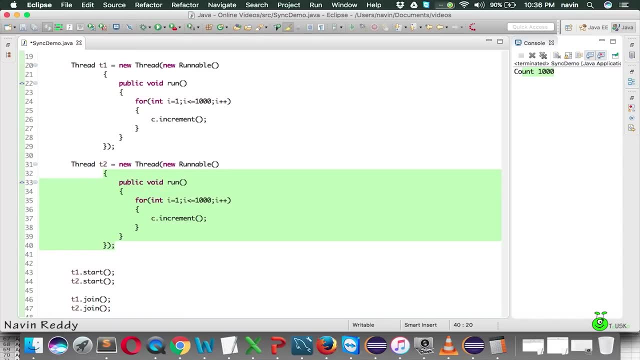 So we will say t2.join. Everything seems good, right? So if you run these two loops, if you run these two threads, it should increment for approximately 2000 times, right? So value of count should be 2000.. 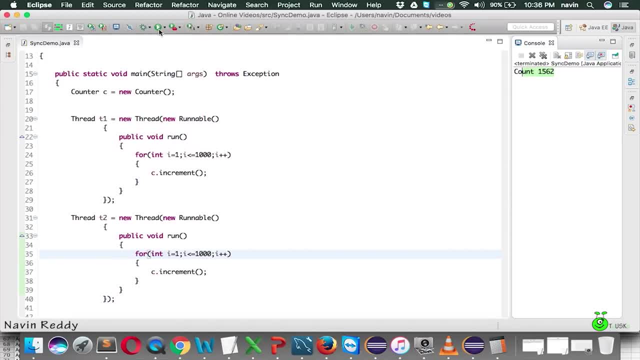 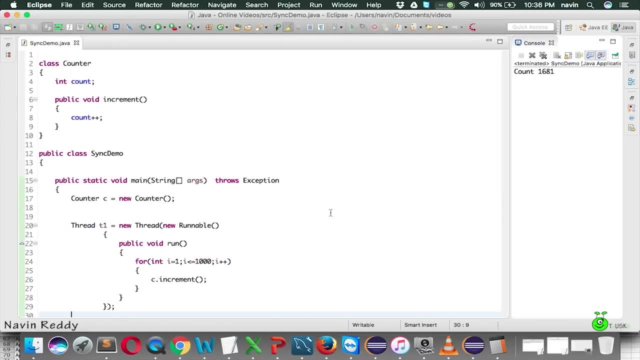 And if we run this code- that's weird- We are not getting 2000.. If we run this once again, we are not getting 2000.. Now why is that the case? It's because when two threads are doing this addition at the same time. 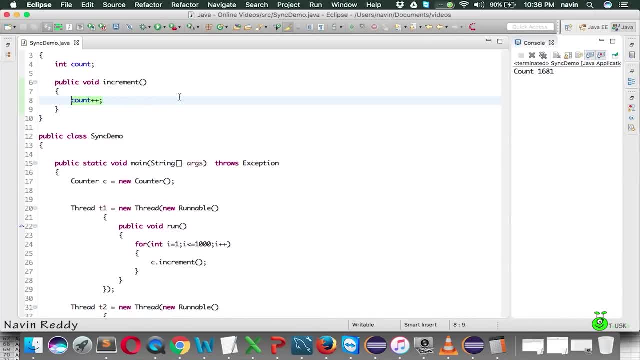 this statement looks very simple. right, This is incrementing the value, But this is not a simple statement. Count++ simply means count equal to count plus 1. That means we are doing two. We are performing two actions here: One is addition and second is assignment. okay, 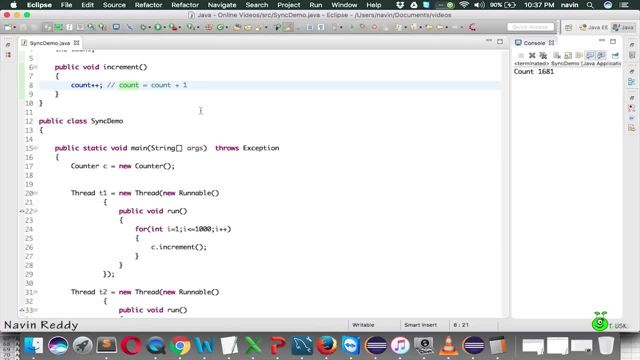 So let's say t1 and t2, they are running in parallel, right? So t1 comes to increment and says: hey, increment, I want to execute. So your increment says, okay, go on. So t1 fetches the value of count, which is 0.. 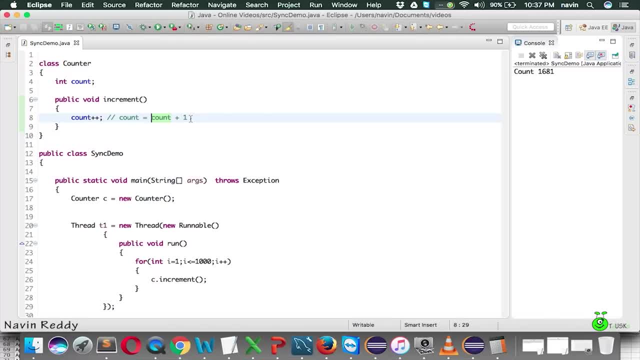 So t1, fetch the value of count, which is 0. It says plus 1.. It is making it 1 now. So the count value for t1. I mean the count value is 1. And you assign the value of 1 to count. 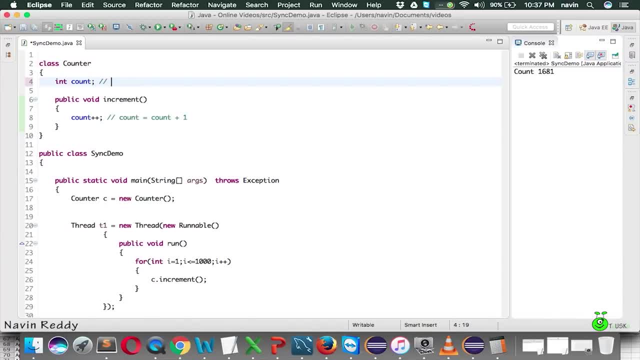 So the current value of count is 1.. Now t2 reaches, t2 says: okay, count, give me your value. Count will say: my value is 1.. t2 will say: okay, your value is 1.. I will add 1.. 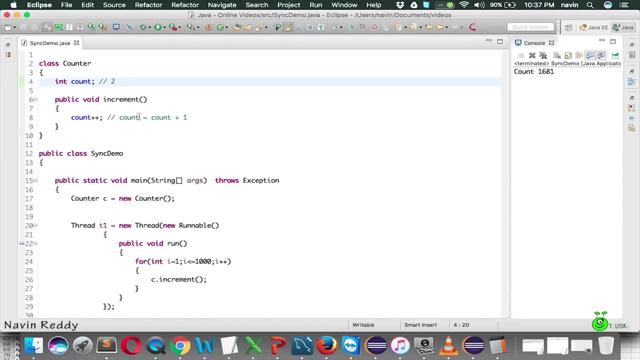 The value of count now is 2, right, So it will assign 2.. Now t1 will again come. It will fetch the value of count, which is 2.. It will assign 1.. The value of count becomes 3.. 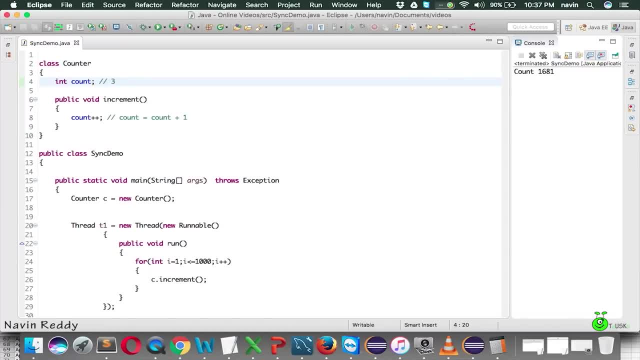 And this goes on right. So for t1 running 4,000 times t2 running 4,000 times, in total it should be 2,000.. But what is happening is somewhere in between, when t1 reaches and asks for the value of count. 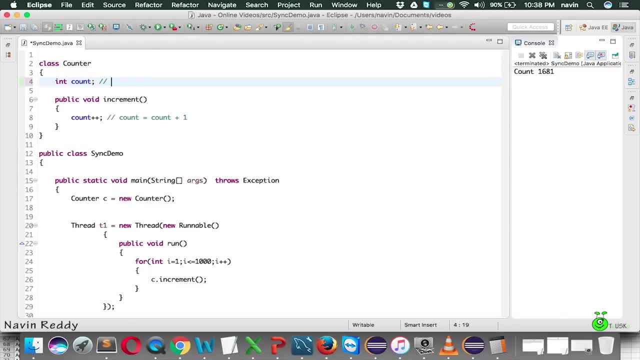 so let's say the current value is, let's say, 600.. So somewhere after 600, t1 reaches and t1 says: hey, count, give me your value. Count says: okay, my value is 600.. By the time t1 is adding the value, 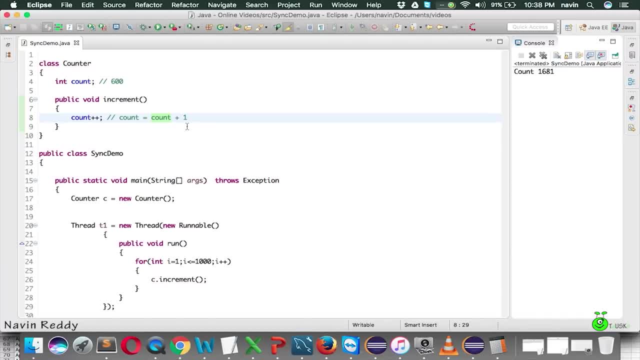 so, by the time t1 is adding the value, what t2 is doing is t2 has also fetched the value of count at the same time. Okay, So both are both have, both are asking for the value, And the value both got is 600.. 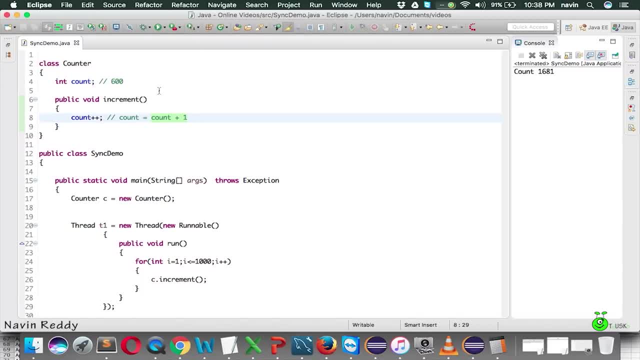 Both has added 1, which is 601.. Because both have 600, both are adding 1.. So they got 600, 1. And that value is assigned to count. So where it should be 2,600, I mean. 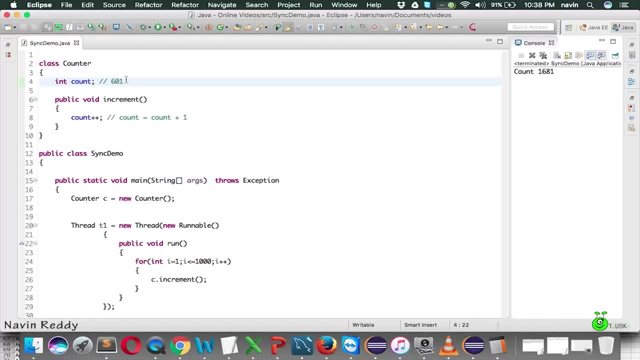 where it should be 600, 2, or 600, 2,, it is 601.. Because, instead of incrementing 2 times, we are incrementing only once, Because both are fetching the value and both are incrementing it at the same time. 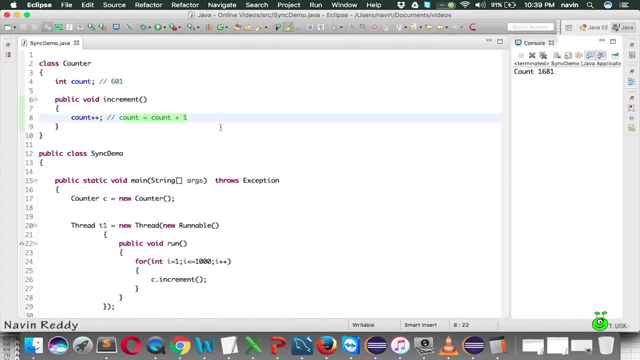 And this is not happening. this is not happening once or twice, It is happening multiple times. That means both this thread are using this method at the same time. That is creating the issue: Both the threads are accessing this method at the same time. 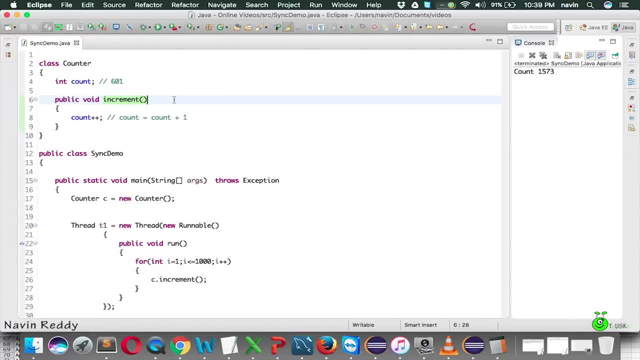 That is what is creating the issue. What I want now is: if t1 is executing the increment method, t2 should not execute this. If t2 is executing this method, t1 should not interfere. That means you want only one thread to work with this method. 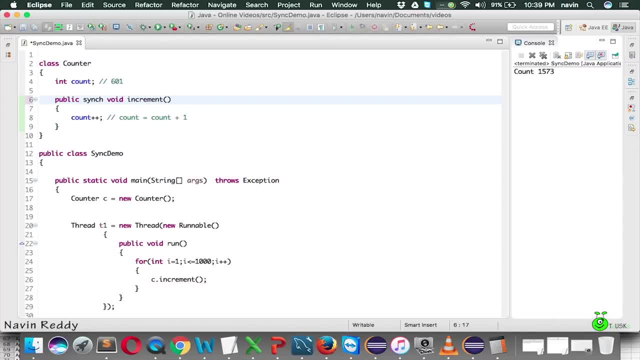 And how to achieve that? If you make this method as synchronized. If you make this method synchronized, that means only one thread can work with this method. If t1 is working with increment, t2 has to wait When t2 is working with the method. 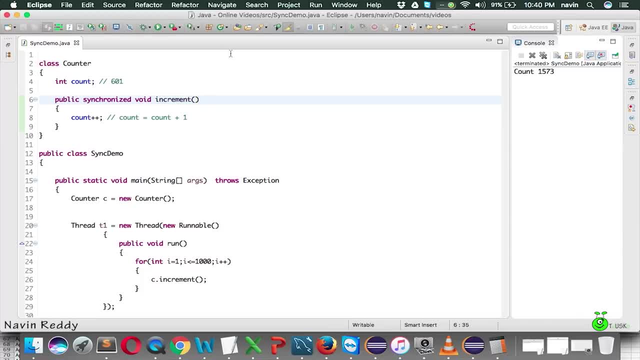 t1 has to wait. So maximum one, only one thread can work with this. So if you run this code now, you can see we got the count value as 2000.. Let me run this once again. You got the value as 2000.. 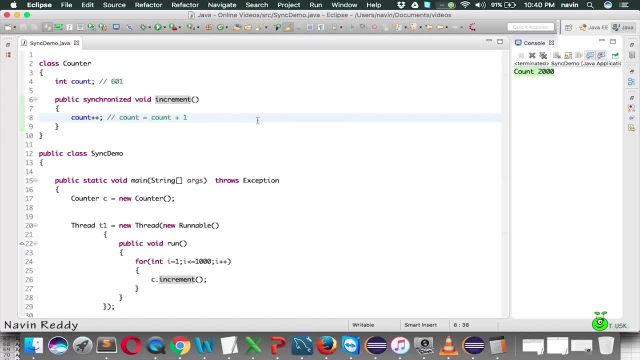 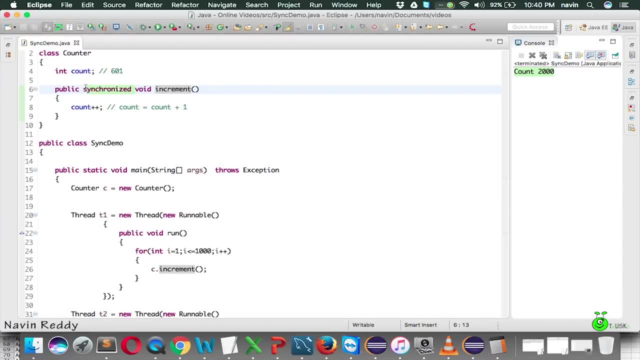 It is that simple. Okay, So that is how you use synchronized method. So point to remember is: when you don't make your method synchronized, that means your method or your object counter is not thread safe, Your class is not thread safe. 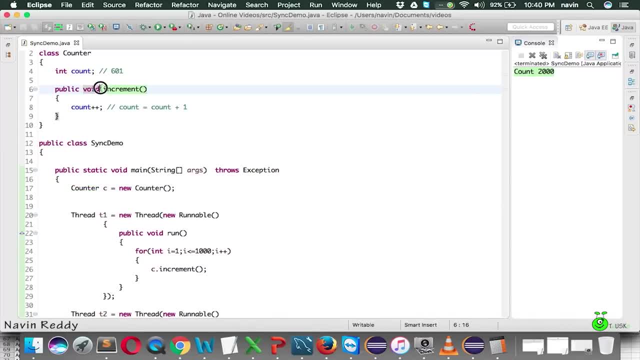 Which means that multiple threads can access the same method at the same time. What we want is we want to make this method synchronized so that only one thread can use it at a time, So when t1 is executing increment, t2 will not interfere. 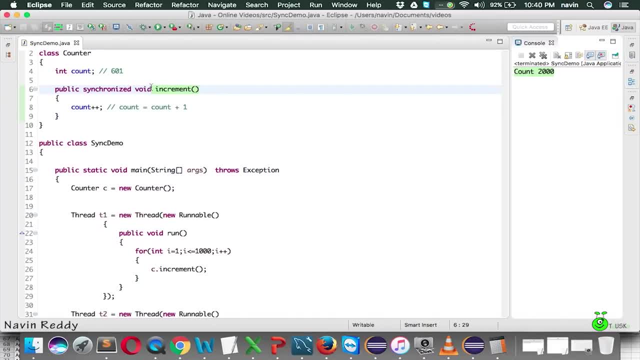 So t2 will wait, And when t2 is executing increment, t1 will wait. So that is the idea behind synchronized methods. Okay, And so once we have talked about synchronized, we can also talk about string builder and string buffer. So in the examining session, 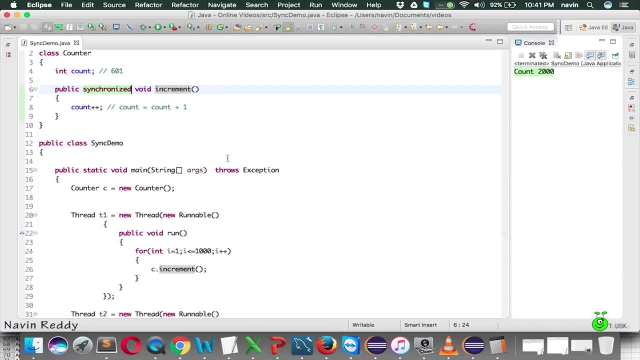 in some next few videos we will also talk about string builder and string buffer. So once we start with string handling, we will talk about that. So that is about synchronized methods, That is about synchronized keywords. Thank you so much. 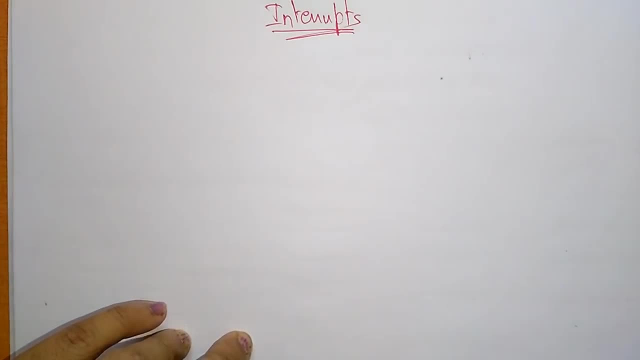 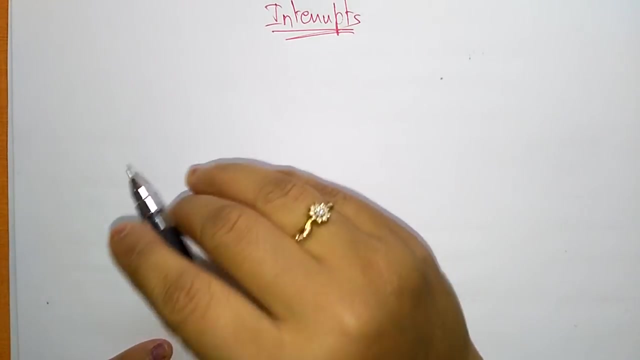 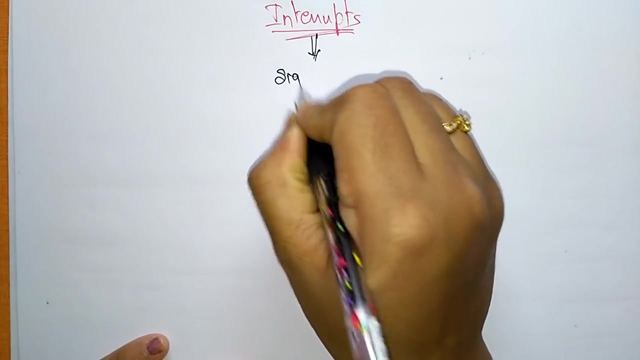 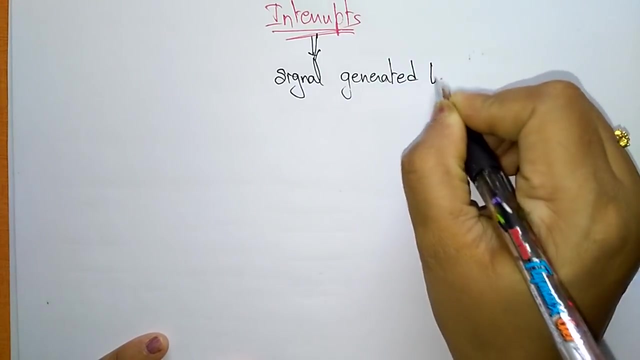 Hi students. coming to the next topic in the subject computer organization and architecture, is interrupts. So interrupts. let us see what is this? interrupts? Interrupts are nothing but a signals generated by the external devices. So it's nothing but a signal. Interrupt is nothing but a signal, that generated by the external devices. 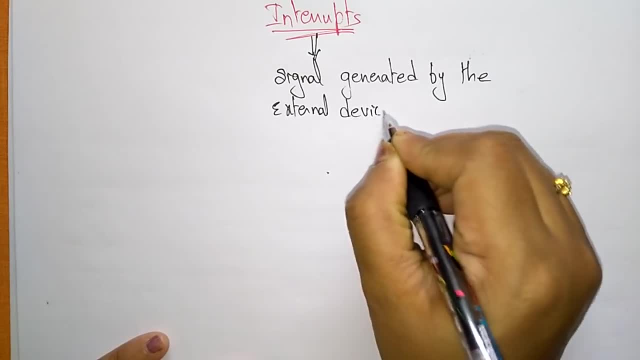 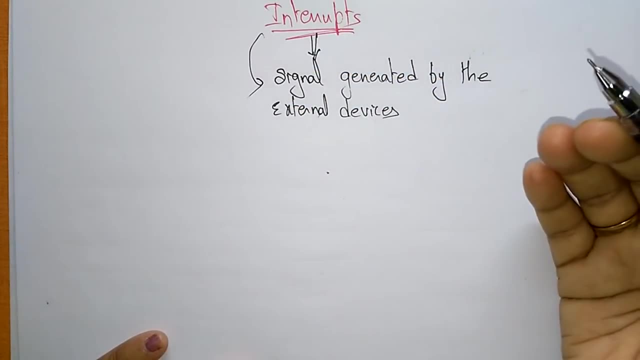 So it's nothing but a signal generated by the external devices. So to request the microprocessor to perform some task means the interrupt signal is asking the microprocessor to generate means to perform some action. So it is a signal given to the microprocessor. 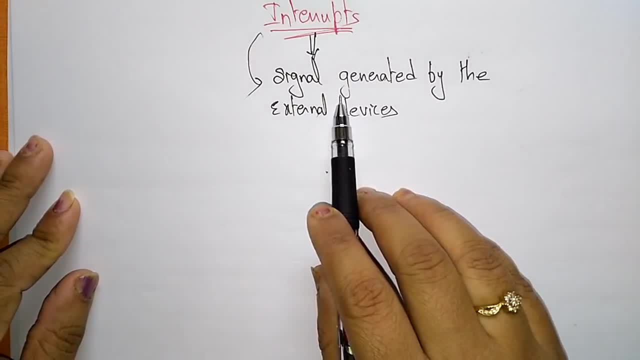 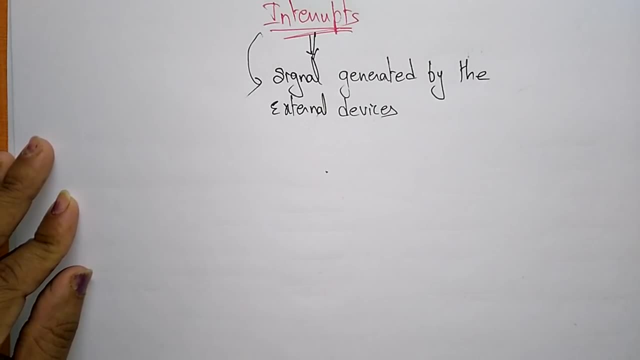 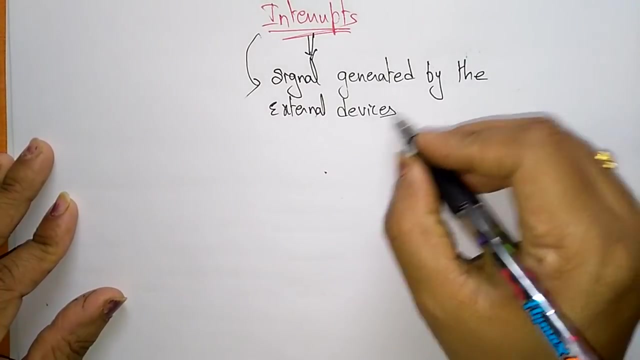 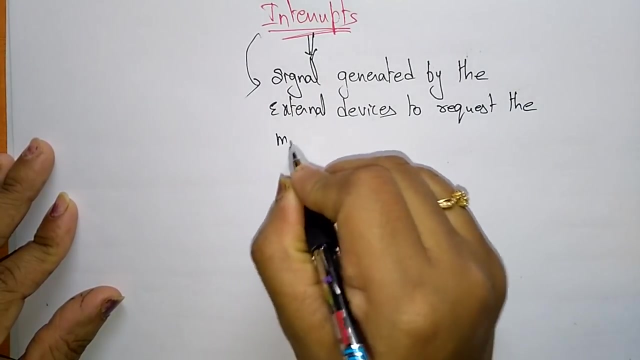 So let me explain again: Interrupts is nothing, but it is a signals generated by the external devices, like all the devices. So let me explain again: Interrupts is nothing, but it is a signals generated by the external devices. So to request the microprocessor to perform some action is asking the microprocessor to generate. means to perform a task, means the interrupt signal is asking the microprocessor to generate. 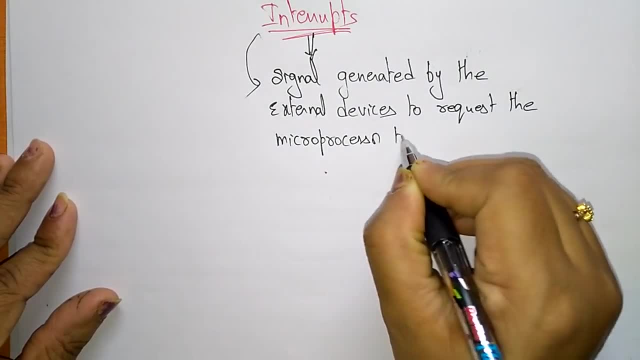 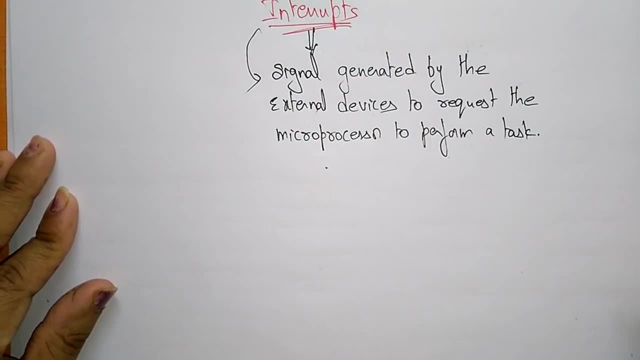 Interrupt signal is asking the microprocessor to perform some action. means the microprocessor to generate means to perform a task. Ok, that is a signal generated by the CPU microwave. using incorrupt signal is asking the microprocessor to perform some action. means the microprocessor should not notice the environment because the Landsat system can read the official data. a Vancouver data right.